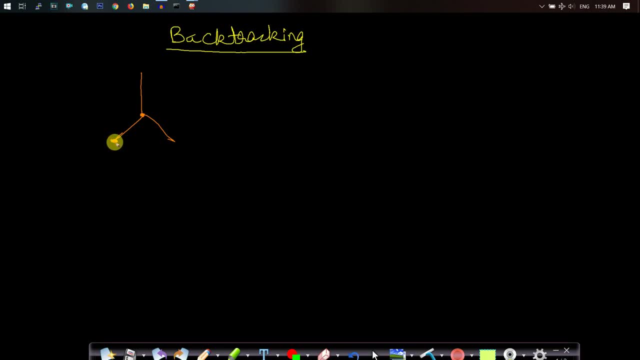 move left or to move right. and there is another point. here again, there are two options. there is another point and you have two options. okay, let me mark. this point says a, b, c, d, e and f, and and here g. okay, and let's say, you want to reach e. this is your goal. okay, this is your goal, you are. 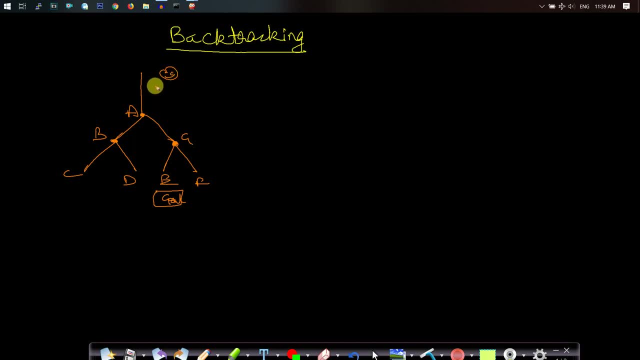 at the starting position. so how will you go if you don't know the way? what you will do is: first you will go this way. okay, and from here you have two options: either to move left or to right. let us say you move left. again, you have two options at b: either to move left or to right. 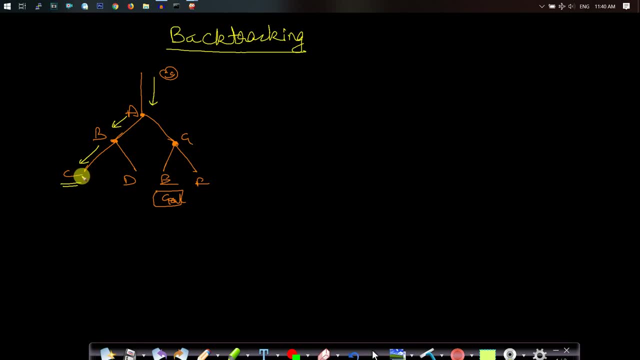 again, you moved left. okay, you reached c and on reaching c, you found out that this was not your goal. then what you will do is you will go back to b and from b you will take the other way. the other way was d. so you went to d and you again found out that this is not your goal as well. 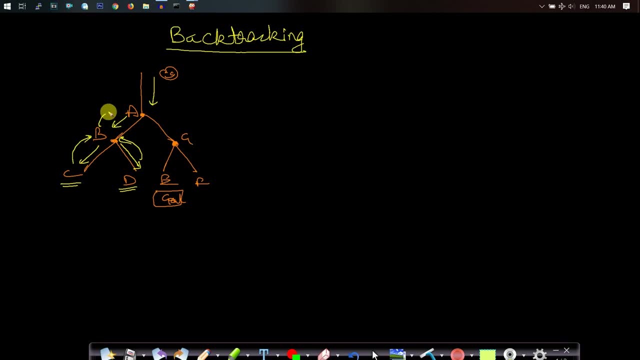 then what you will do is you will go back to b, and from b you will go back to a, and after reaching a, you know that the left side of a will not suffice your goal, so what you will do is you will move to the right side, so you will go to g. from g, you have 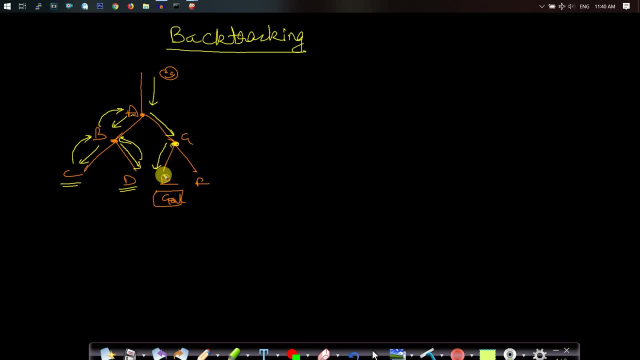 two options: either to move left or right. let us say you moved left and you found your goal. okay. on reaching c, you found your goal, not c, but e, this is e. on reaching e, you found your goal. then what you will do is your program has succeeded and it will return true or found, or will print the value. 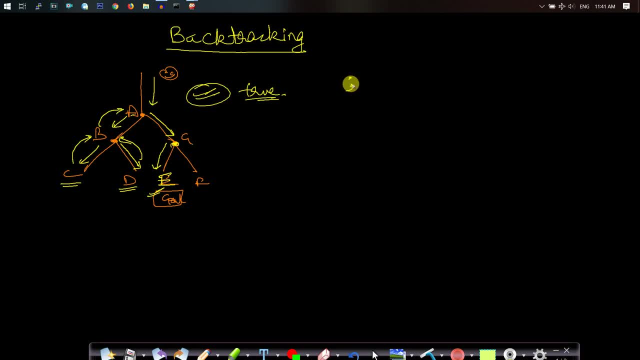 okay, in prologue you have something known as a semicolon. okay, what semicolon will do is it triggers further solution. so if we give a full stop, then this goal will end here and nothing more will be done. but if you give semicolon, then further goals will be searched and again you will. 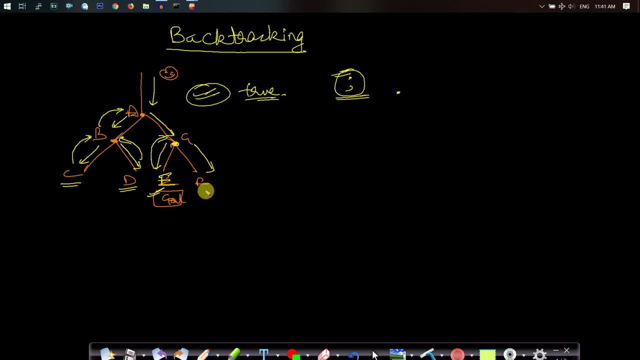 move back from e to g and will go to f and we'll see that there is no goal. and again, from f you will go to g. there is no other way. you have searched both the ways, so we you will move back to a and you have also searched both the. 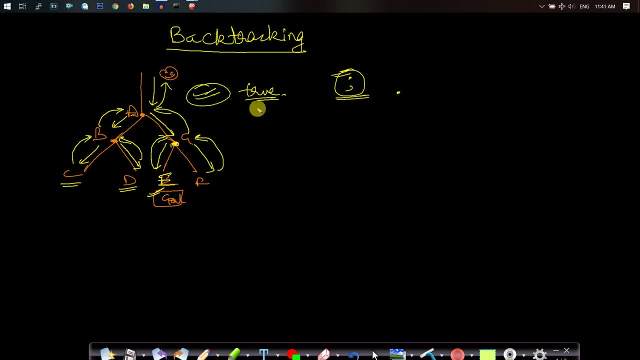 ways from a, so you will move back, okay, and then you will return as false. so once you had returned true, because you found your goal okay, and if you give a full stop, then it will end here. so this is just like c plus plus, where if the goal is found, you will stop. okay. let us see this backtracking by. 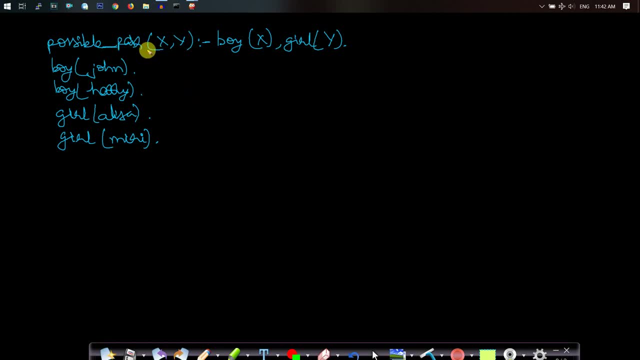 using an example. okay, so i have taken an example where we will form pairs. the pair will consist of x and y, where x will be a boy and y will be a girl. okay, so can you predict the output? these are the boys and these are the girls. these are facts, okay, and this is a rule. 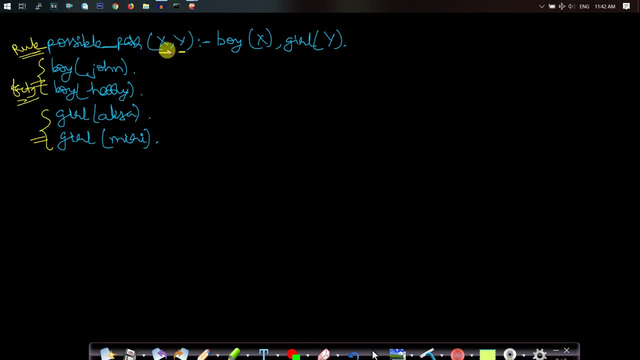 so this rule says that we can form a pair if, provided, x is a boy and y is a girl. so how will the output look like? the output will be first: x will be equals to john. okay, so let me not tell you first about the output. let me draw the structure. okay, so what will be done is this: 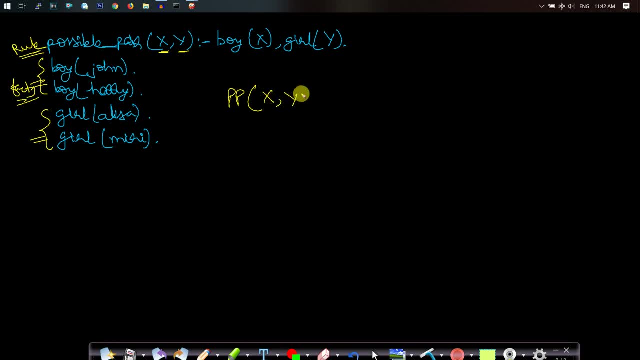 function possible pair will be called on x and y. let us say we called on x and y, then what will be done is we will have two options for boys. this is a condition one, this is a condition two. so for the condition one, we will have two options: boy, john or boy. we have harry, okay, so we have two. 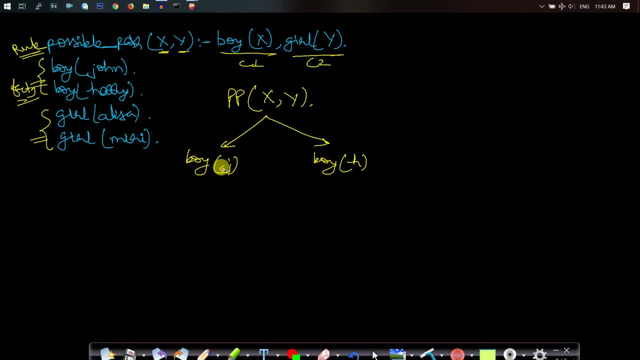 options: boy john or boy harry. then for each boy, for each boy, for each x, you will have two options for girls: girl elisa, girl miri, okay. and for each uh, for each option of harry, you will have again girl elisa and girl miri, okay. so you can see that first when you write the query, as possible pair. 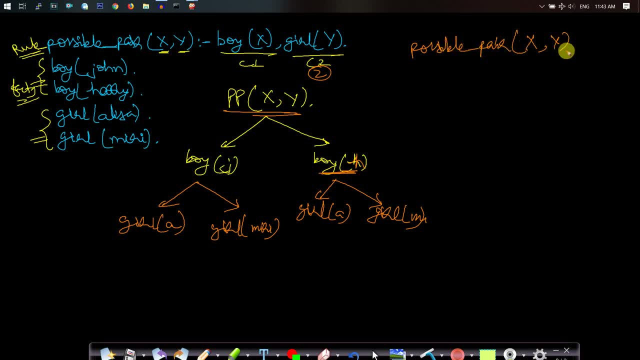 x comma y, in order to find what are, what are my possible pairs of groups which can be found. then what it will do is, internally, it will follow a tree like structure, and it will start from this possible pair x comma y, then it will go to our 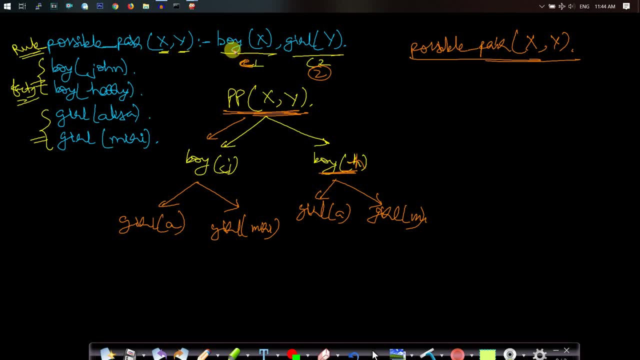 first query, not the first query, but the first condition. the first condition is boy x and it will match with john because this is first in our order. okay, john comes first, before harry, so john will be run first and then x will be assigned to john. okay, and then we will come to y for john. we will run this girl y. elisa is first, and so it will be. 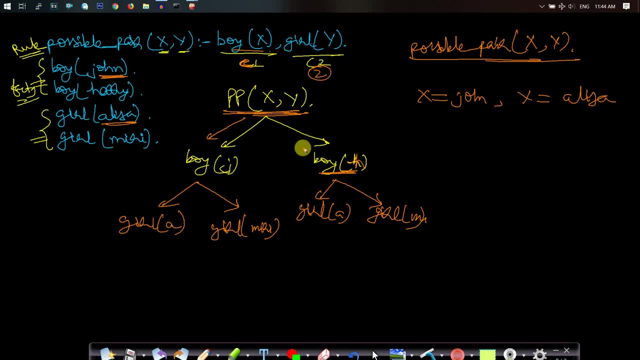 run first and y will be assigned to elisa first. then what will be done is it will be x will be john and y will be elisa. after doing this, it will go back to john, okay, and x is john now and y will be the right path. 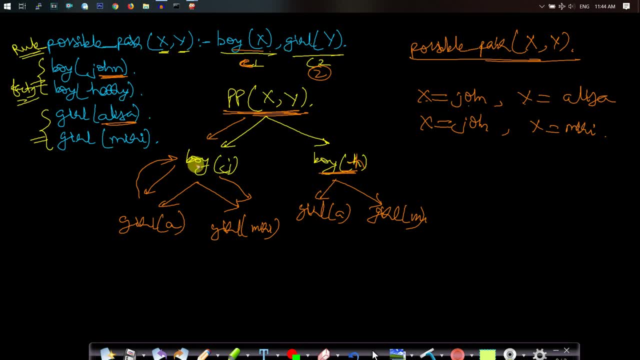 will be miri. okay, so it will take all the possible values for john and after taking all the possible values for john, it will again go back to john and since we have traversed all the paths, so it will go back to our possible pair x comma y. now, after going back to possible pair x comma y, 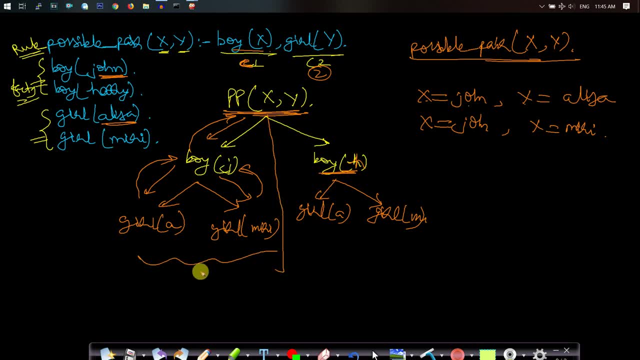 we know that this left part have been traversed, this left part have been traversed, so what we will do is we will move to the right part. so this is our right part. okay, so the right part contains another boy named harry. so this is done, so this boy will go to harry. so x will be initialized with. 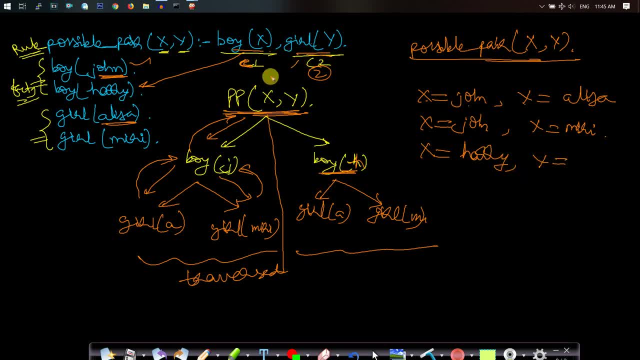 harry, and then we will move to the girl, and from girl you can see that elisa comes first. okay, elisa comes first. so this y will be initialized to elisa first, and after printing this elisa, it will go back to boy and then it will come again to the second girl, which 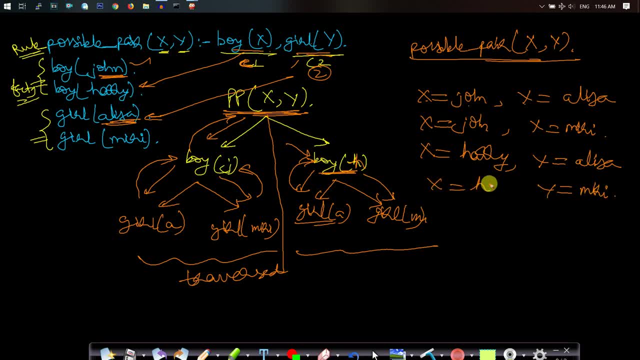 is miri now. y will be initialized to miri, x will remain the same as harry, okay, and after traversing all the possible values for harry, it will go back to harry and there is no other option for harry. so it will go back to possible pair and you can see that all the possible conditions. 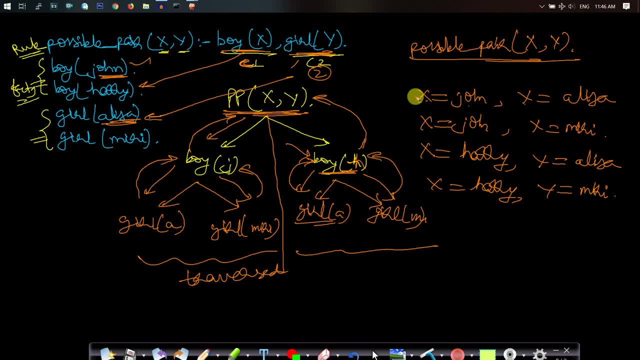 boy and girl have been traversed, the entire tree is traversed, and so this is our output, starting from x equals to john and y equals to elisa, to x equals to harry and y equals to miri. okay, so this is a very beautiful example of backtracking. 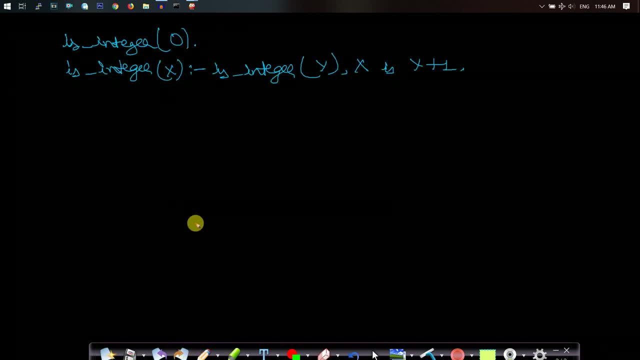 in prologue. let us see one another example, and this example is a trickier one. okay, so let us say we write: is integer 0 and is integer x, is integer y, comma x is y plus 1. so if you give the query as is integer 0, then it will come out to be true, because this is our. 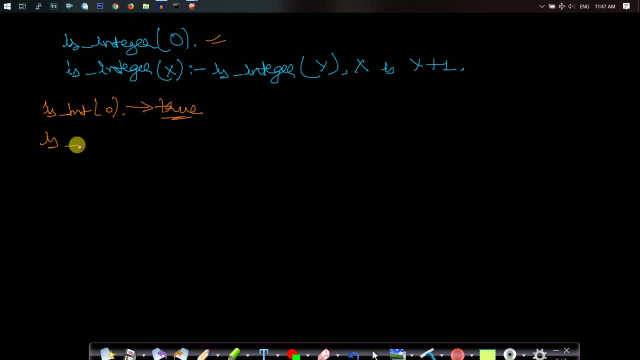 fact here. okay, but if you give some another query, let's say, is integer 2, then this will also come out to be true. but this will not directly be sufficed by this condition, but it will run starting from this condition. okay. so let us draw another tree. structure is integer 2. 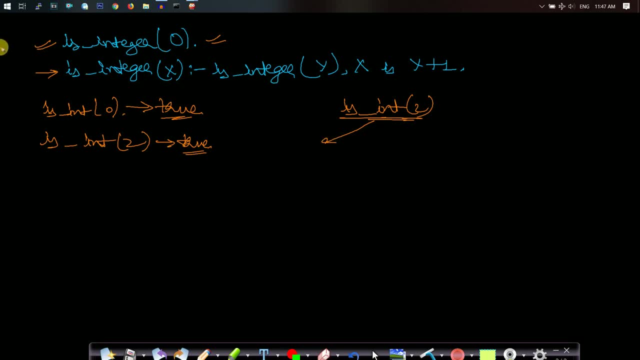 now, from this part, we will have two conditions. let us say this is l1. let us say this is l2. okay, this will have two conditions. let's say it is matched with is integer 0 and it can even match with is integer x. okay, so, since this is true, this will be false because the value here is not 0, but 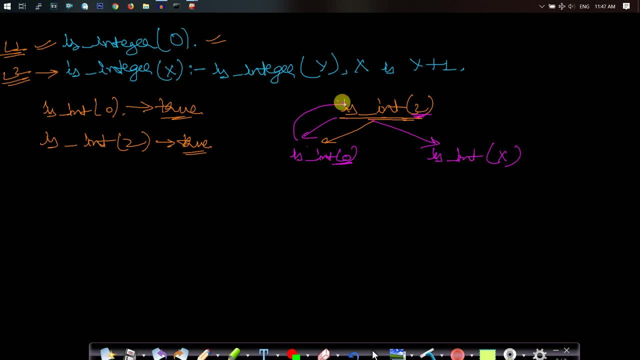 2, so it will take this path and again return to 0 and it will return to 0 and it will return to back and take this path. okay, so here y, whatever y is returned, x will be initialized to y plus 1. okay, x will be initialized to y plus 1. you can see that x is y plus 1 and now from here we will. 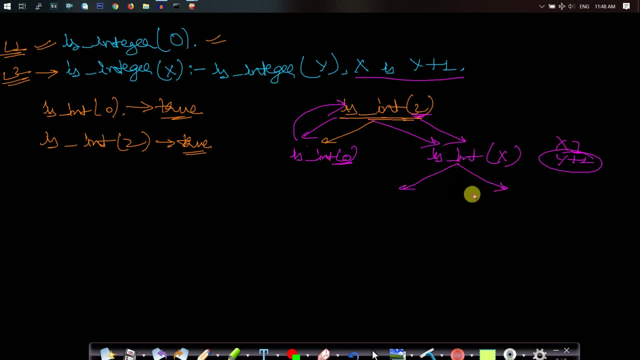 be having two branching. okay, with, two branching will be there. the first one will be initializing: x equals to y plus 1, and the second one will be for is integer 0 and the second one will be for is integer x. okay, these two options will be run. so when we run, the first condition is integer 0. 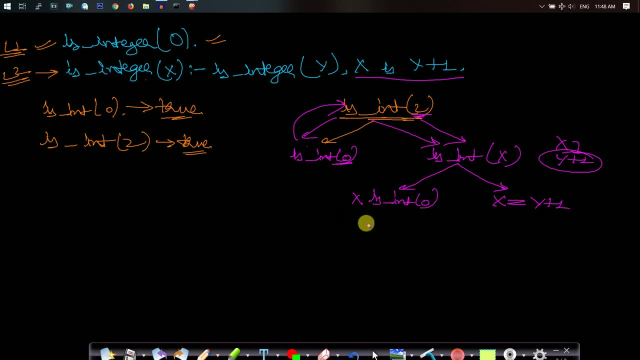 this will fail. okay, and so the second one will run. the second one is: is integer x? okay, again, it has two parts. x is equals to y plus 1. okay, here x's value was 2 and here x's value will be 1. okay, again, like this. we will have another option. okay, so we will have two parts. x is equal to y plus 1. 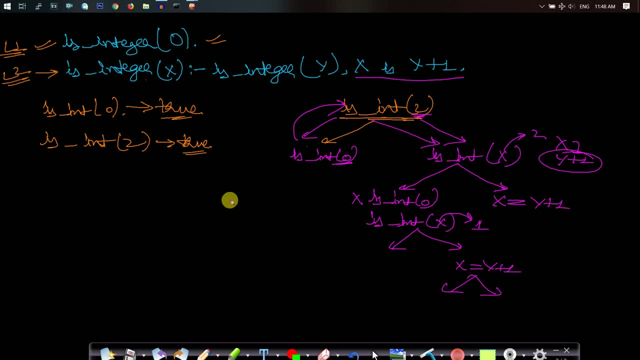 okay, and this will go on until we reach the condition where x is equals to 0, and so this value will be returned and one will be added each time. one will be added each time and finally we will get the result to be true. okay, and if you give, say, an integer value, let us say you gave. 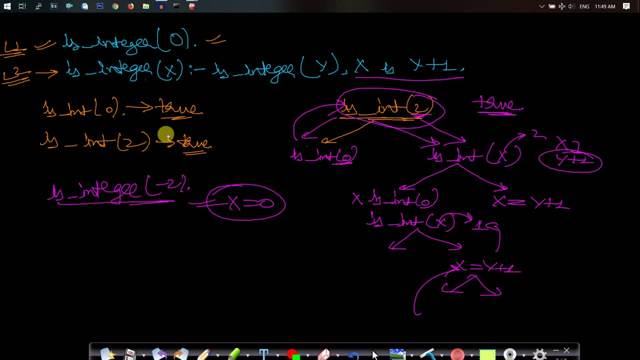 is integer minus 2, then this won't run, because this, because this condition is saying that y's value will be x minus 1. okay, so whenever give, whenever we give any query, then it will keep decreasing the value and our stopping condition here is is integer 0, so whatever. 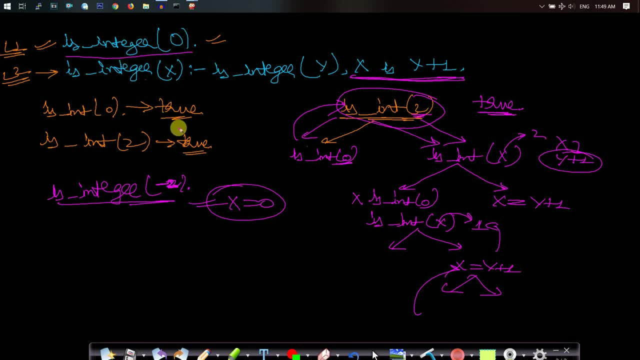 value we give with below 0 will fall into an infinite for loop- okay, infinite loop and it will not run until the stack gets empty. okay, so you can see that I have written a code for it. let us see the code first. so let me open the code. so this is our code: I. 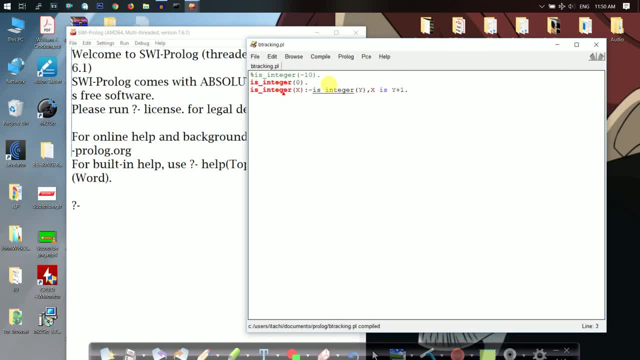 hope you are able to see it. you can see that this is: is integer 0. okay, I have written the same two lines and let us run it for some positive values. so let us say we run for is integer 2, then what is done is true, is returned. and if I give a semicolon, 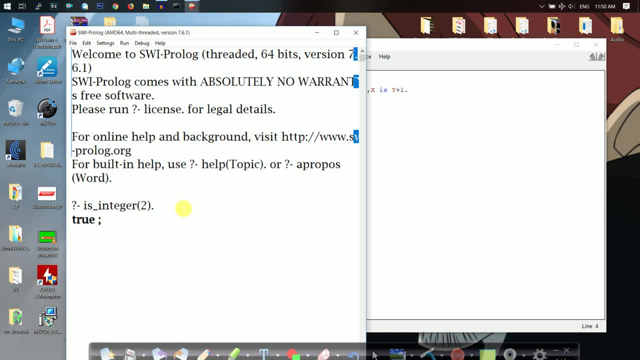 then it will fall into an infinite loop and you can see that nothing is being returned. you will have to press ctrl c and then abort. why? why it is falling into an infinite loop is that when we already reach 0, then after that it is searching for the values less than 0 and there is no stopping. 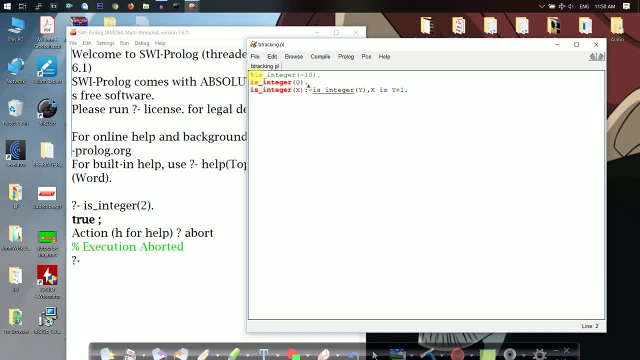 condition here below 0, so it will not stop, okay. so if I just uncomment this line is integer minus 10, then you will find that two times, two times this uh value will be returned. means two, two times true will be returned. so let us see. you can see that first. true is for is integer zero this line, okay.